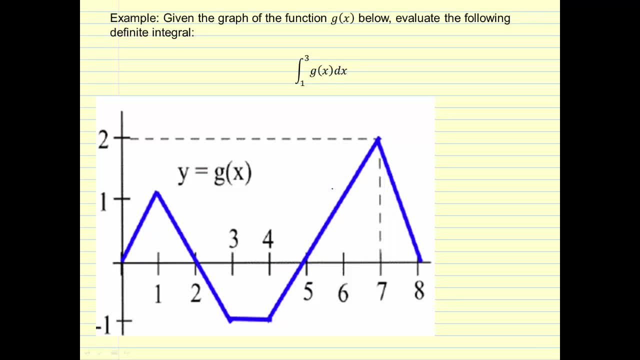 right here, this blue line, It's some random graph of a function And we are asked to evaluate this definite integral. And what I mean by a definite integral is it's basically got this integration symbol and then we've got these numbers that are called the limits of. 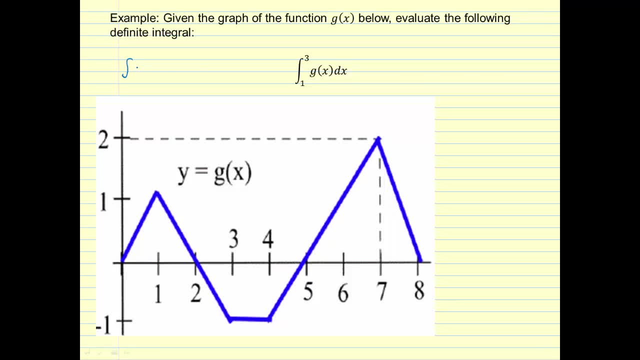 integration If I had just the integral symbol and no numbers. that's called an indefinite integral and that would be a slightly different kind of thing. So for now, what we're basically looking for is how do we find some answer of this definite? 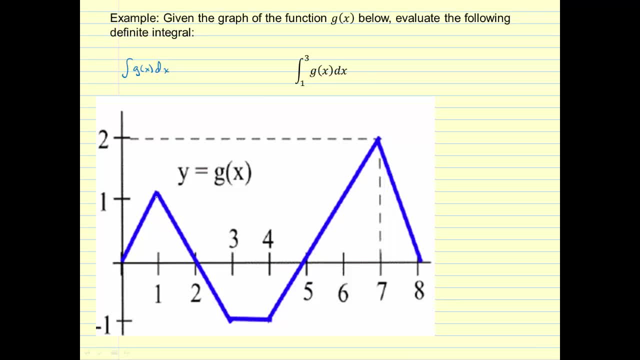 integral from one to three. So the idea here is this can be represented by the area of a region And this region goes from one up to three because we have from one to three And it's the area between the graph and the actual integral. So we're going to go over 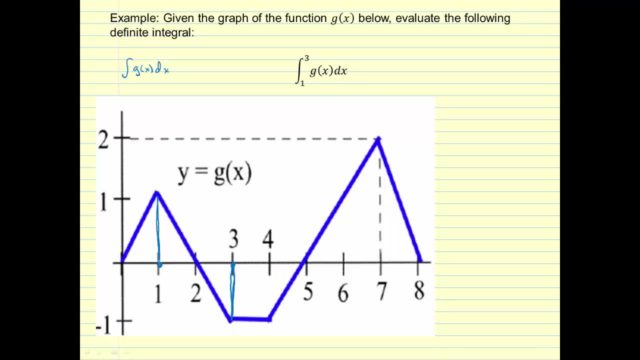 this integral across the screen. And this integral ger one. Now, in this case I'm situation �� From the graph to the excepts to the recommendation from two to three, you can have the compound for that integral in a second. The final 맞 бы light value up to two. 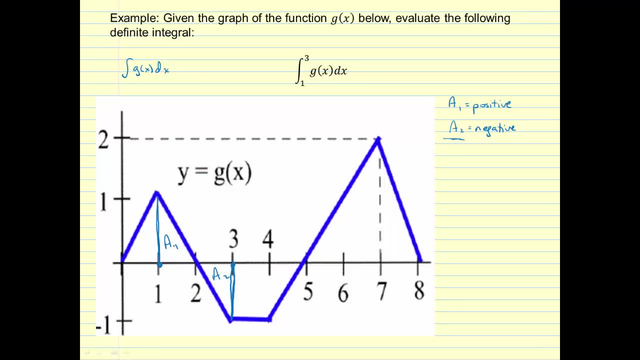 And so you can have a value. So if you're looking at the matrix like this, you can have from two to three And then from this max, two over one over two, You can have anything doing some evaluation. it helps to break it up into different pieces that are above and. 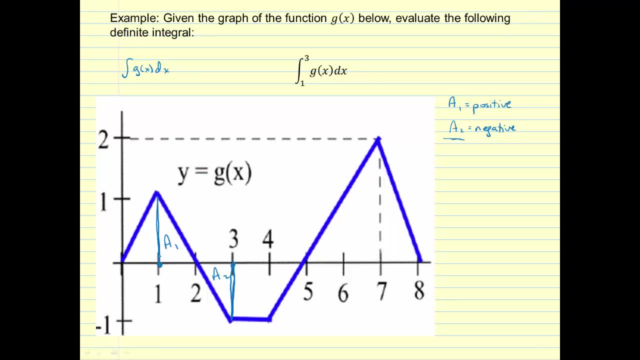 below the axis. So basically, this is a simple formula for a triangle. The area of a triangle, A1, is equal to 1 half base times height, and the base is equal to 1, and the height here is also 1,. so we have 1 half 1 times 1,, which is simply 1 half. That's the A1. 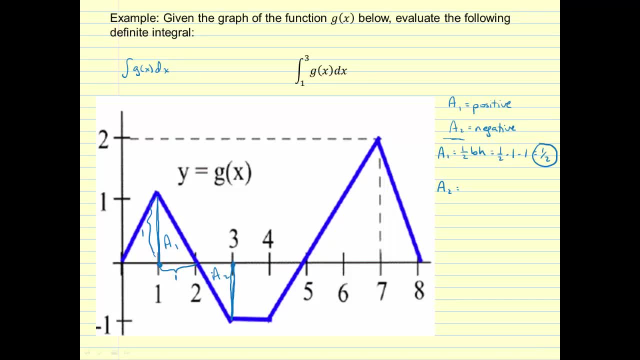 A2, in this case, which is going to be negative because it's below the x-axis. it's got the same base of 1, and the same height of 1, so it's going to be negative 1 half.